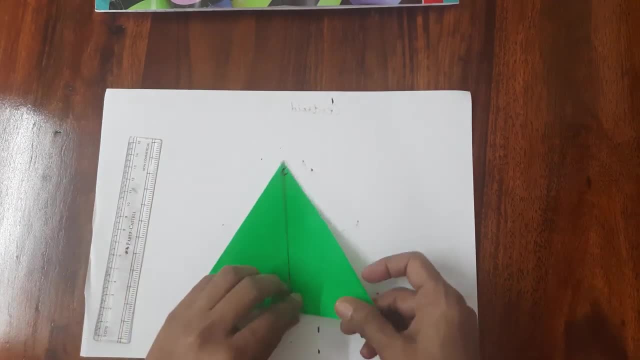 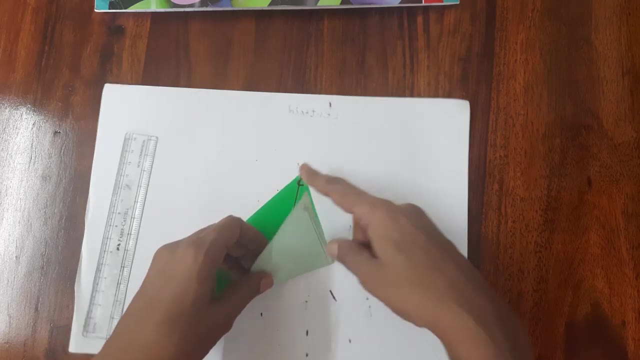 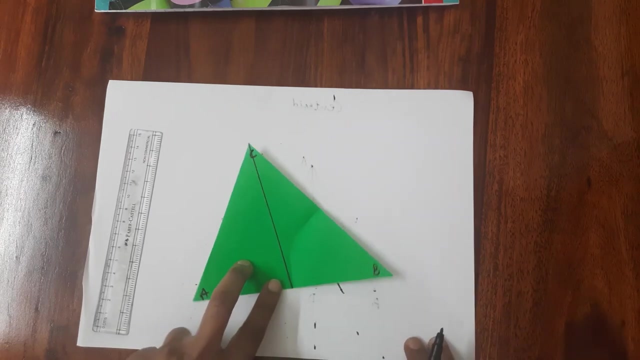 you will get the CPAradial segment. This is called the median. So let us get the midpoint of BC. with the paper folding activity, This side is dividing into two parts, right? So this is the midpoint. So now BC line segment is divided into two parts: B, let us name This. midpoint is D. 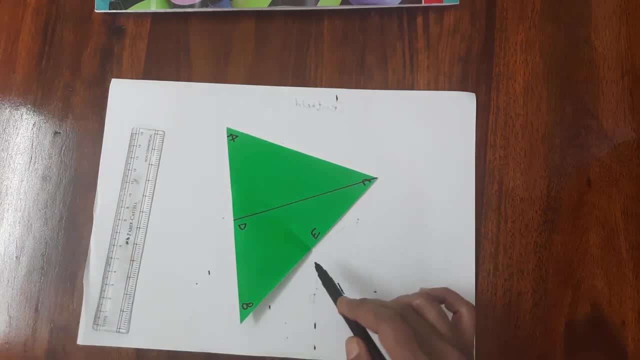 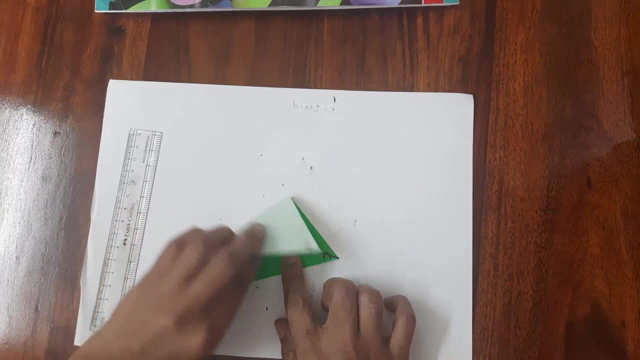 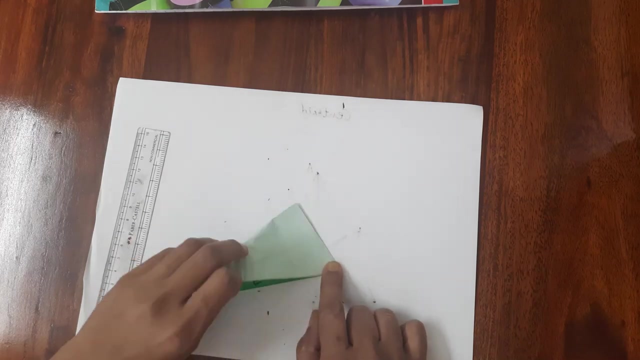 And this midpoint let us name as E. So BE is equals to EC. So same way, let us get the midpoint of B, AC, with the folding of the paper, this and then making a crease here, and we have got point midpoint of AC. so now, 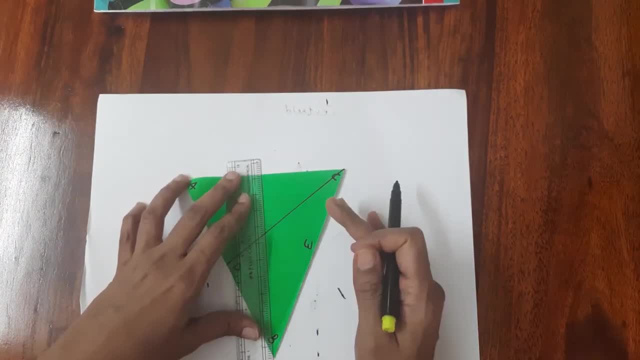 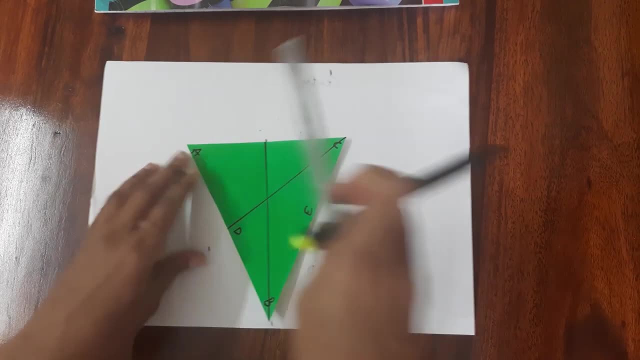 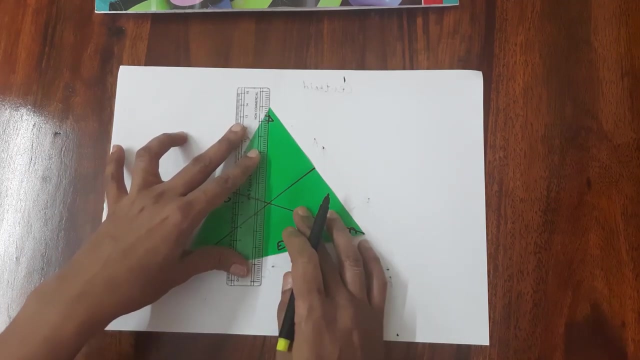 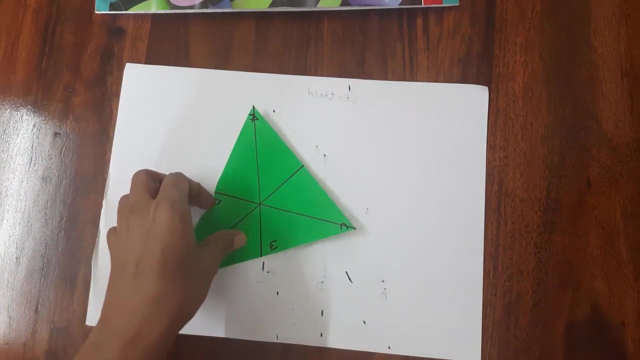 let us join this midpoint with the opposite vertex B, using the scale. same way. let us join now midpoint this E. we will join it with the opposite vertex a. so we have got the three medians of this triangle. this is a triangle right, this ABC triangle, and we have got the three. 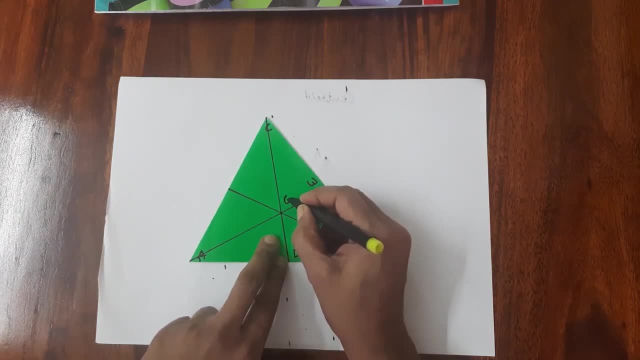 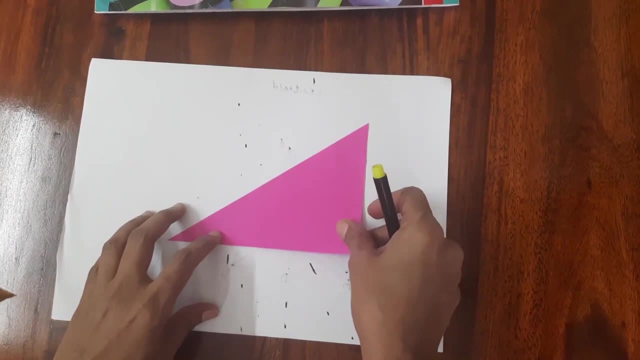 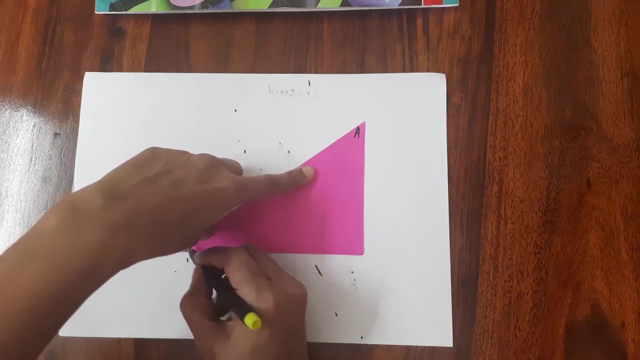 medians. this point of intersection of these three medians is called the centroid of a triangle. now let us see what about the right angle triangle. in case of the right angle triangle, if you this is a, this point is B and here we have C. now, first let us find the 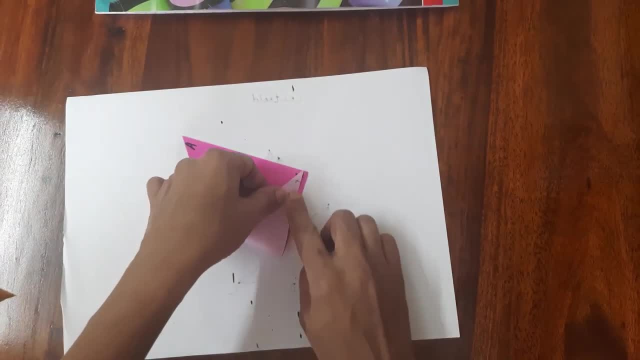 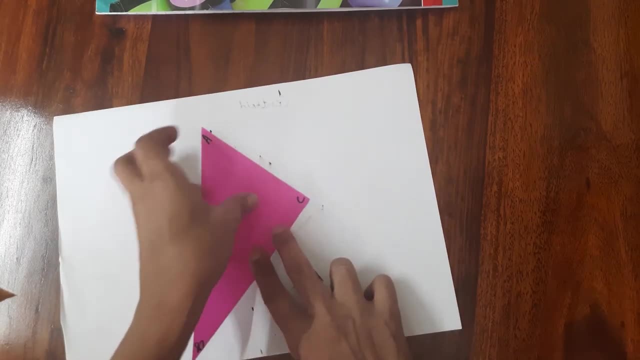 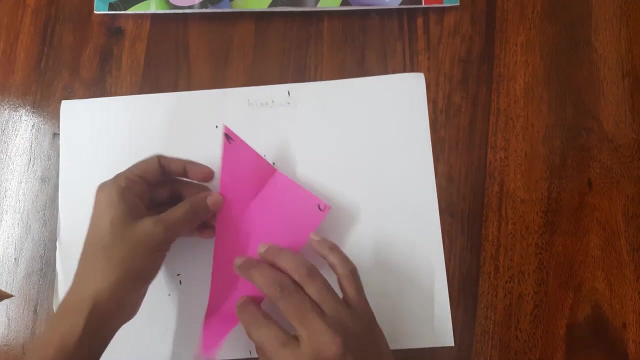 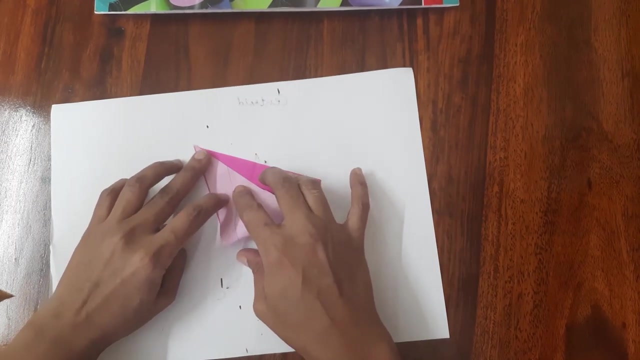 midpoint of all the three sides by folding the paper and making a crease here. so this is a midpoint. now, if you will fold the paper along AC, here you are getting a crease. then, folding along a, B, just join the corners properly and then make a crease. now we have got a three. 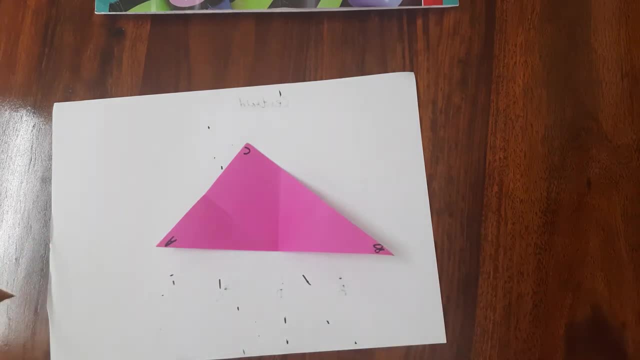 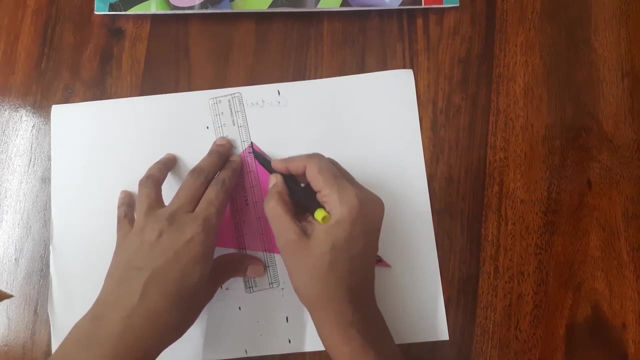 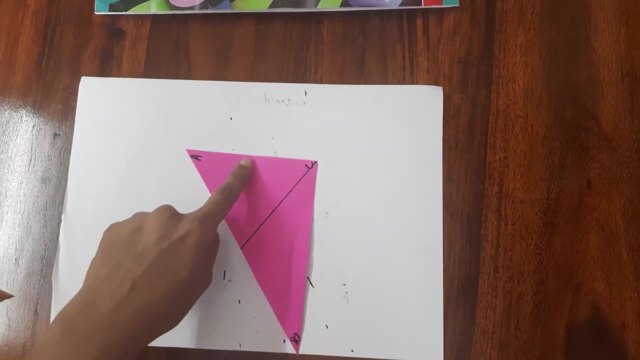 midpoints of these three line segments. so if you are joining these three midpoints opposite to the, to the opposite vertex, we'll get the median of the triangle. this is a first median of the triangle, and then this line segment. this is a midpoint, and here we are having 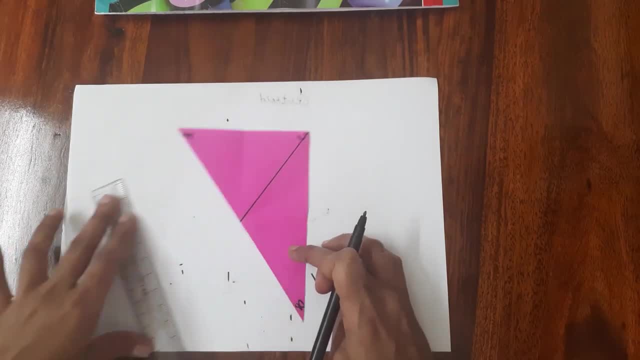 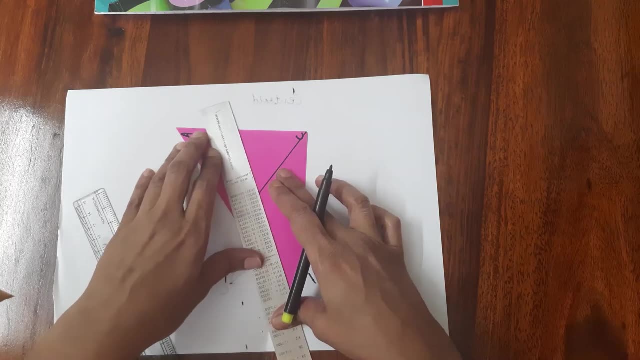 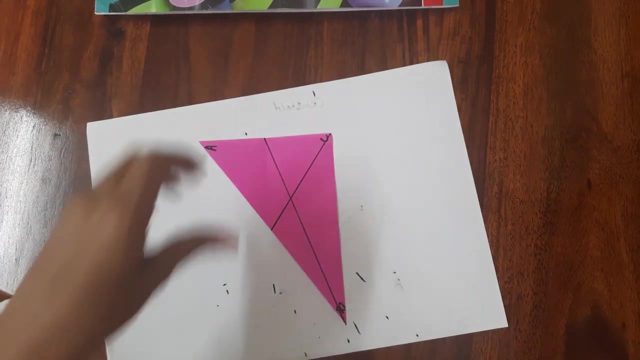 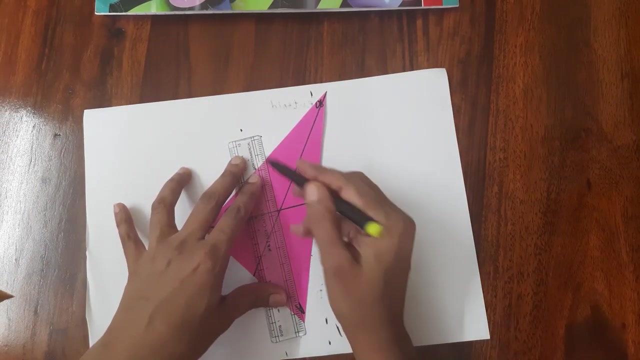 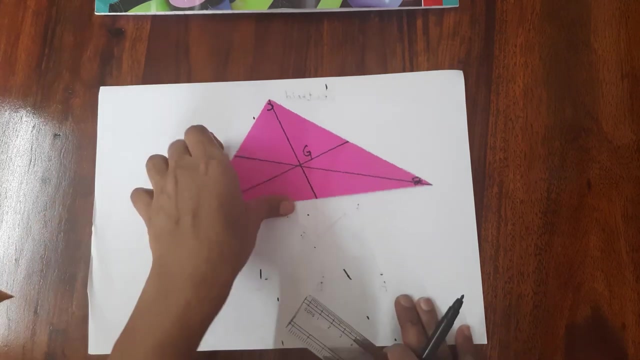 the opposite vertex this. so let us join with the opposite vertex. So this is another median. Same way, we are having this midpoint with this opposite vertex. Yes, So here we have got the median centroid of right angle triangle right. So this was the. it is a right angle triangle, Centroid of a right. 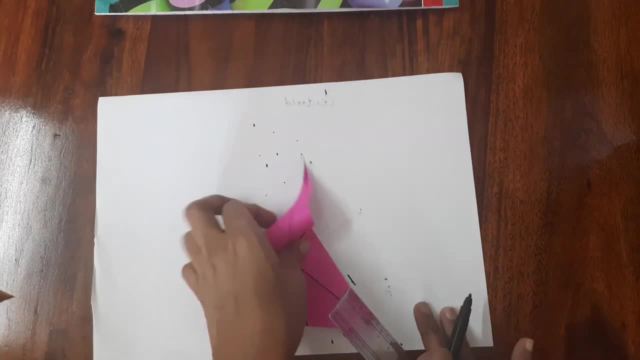 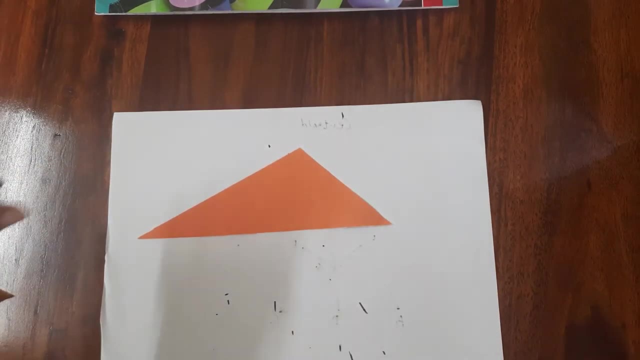 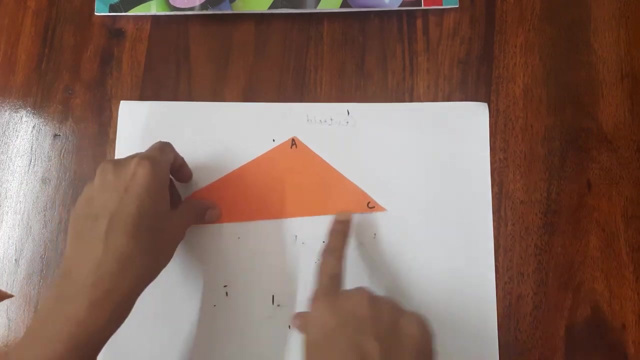 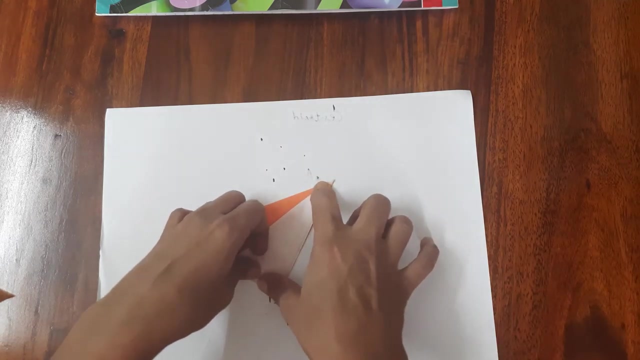 angle triangle also lies inside the circle. So now let us find out the centroid of a obtuse angle triangle. So same way. first let us name the triangle ABC. Then what is the midpoint of BC? We will get it by joining this side, the two opposite, two vertex and 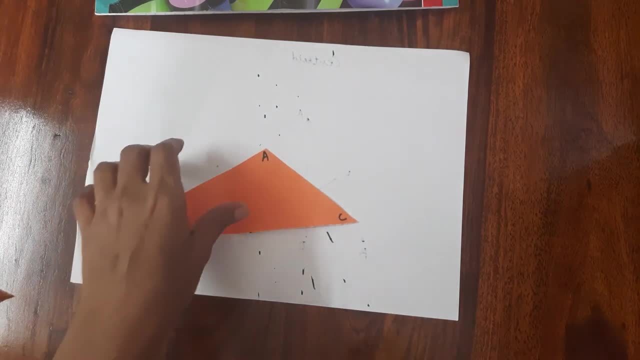 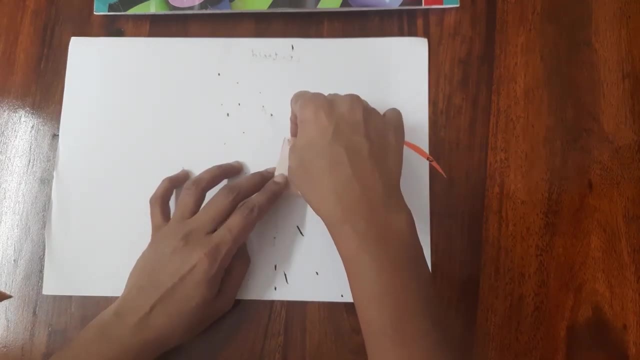 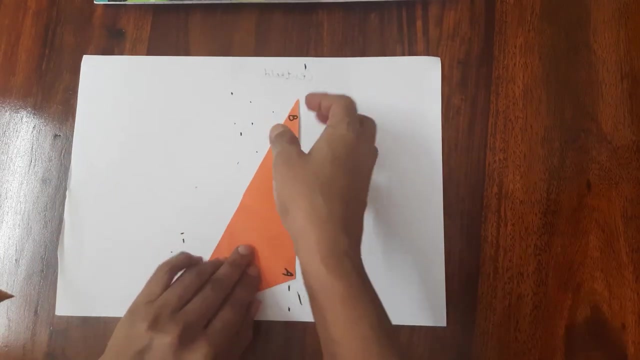 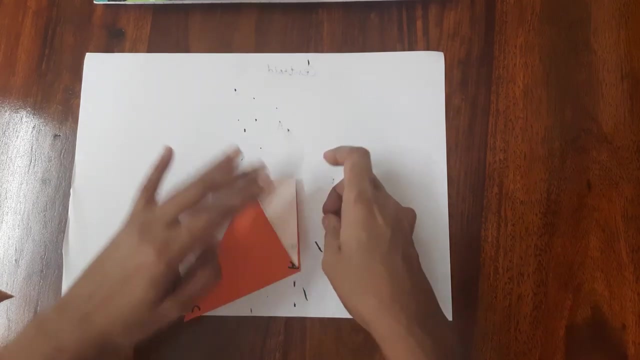 here we are getting a midpoint, Same way A and C. So joining A and C Here it is a midpoint, and then A and B- this side we have got a midpoint here. So we have got a three midpoint. Now let us join the midpoints. 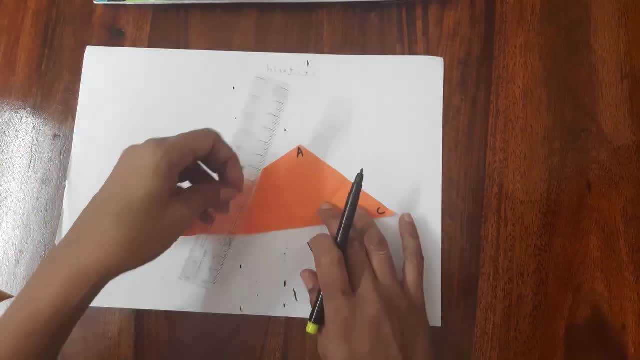 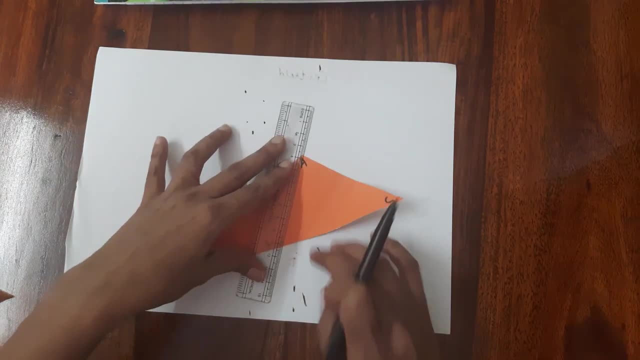 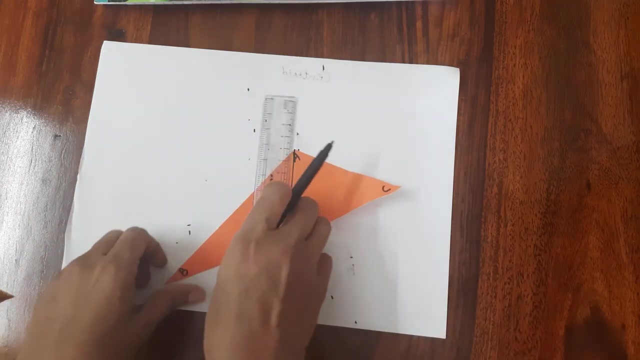 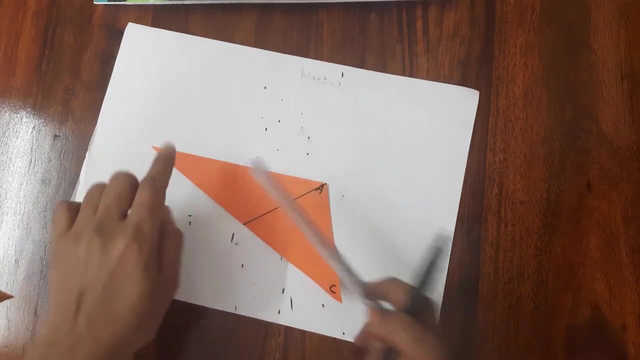 So midpoint of BC is here. It was here. let me see one more. Yeah, this is the midpoint of BC, So let us join it with the opposite vertex. Then midpoint of AB is this is on this crease. So what is the opposite vertex of AB? This C. So let us join it with C. 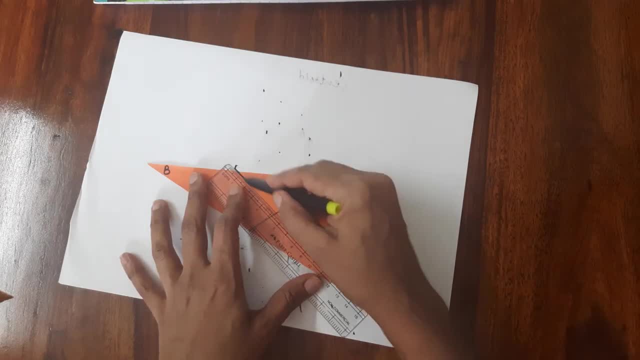 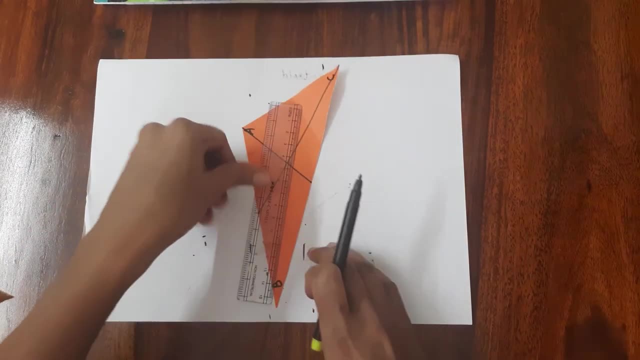 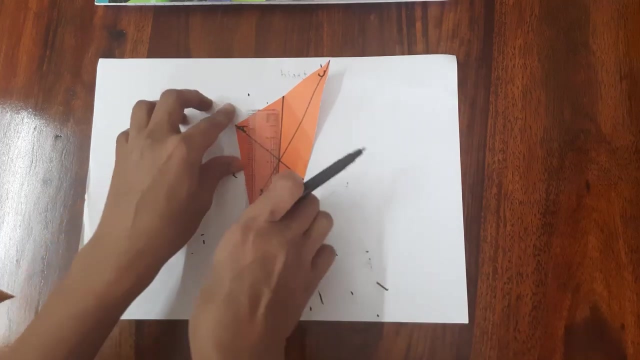 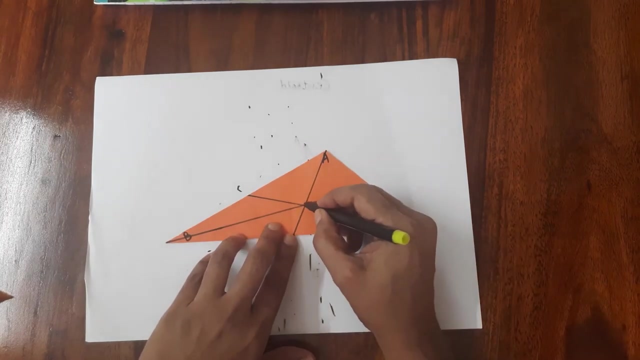 Same way, the midpoint on AC, the crease is here, So let us join this also with the opposite vertex, So where these three medians are meeting, the point of intersection of these three medians here. So this point is called the centroid of a triangle. So what did we?